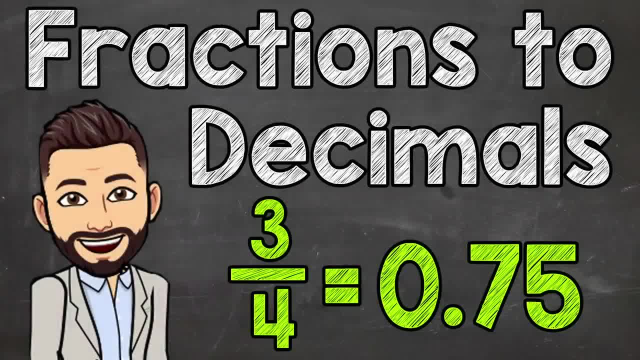 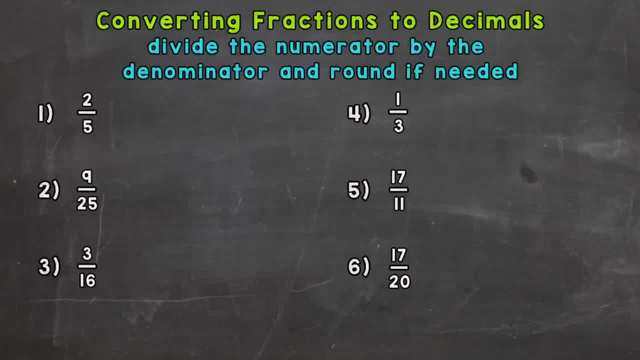 Welcome to Math with Mr J. In this video I'm going to show you how to convert a fraction to a decimal, And if you take a look at the top of your screen, it says: divide the numerator by the denominator and round if needed. So that's exactly what we are going to do. Now I'm going to do a few. 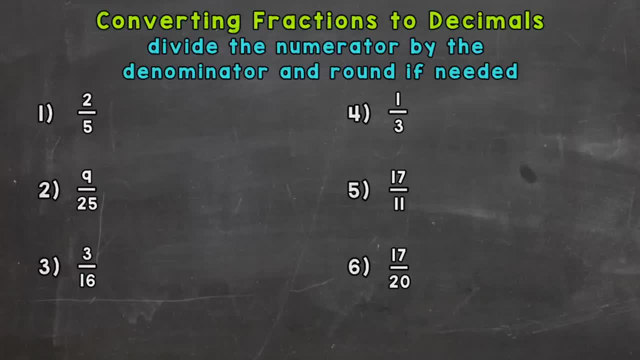 of these by hand, a long division problem to show you exactly what's going on, And then the others. I will give you the answer that a calculator will give you and show you how to interpret everything. So let's jump right into number one, where we have two-fifths or two over five. So here again, 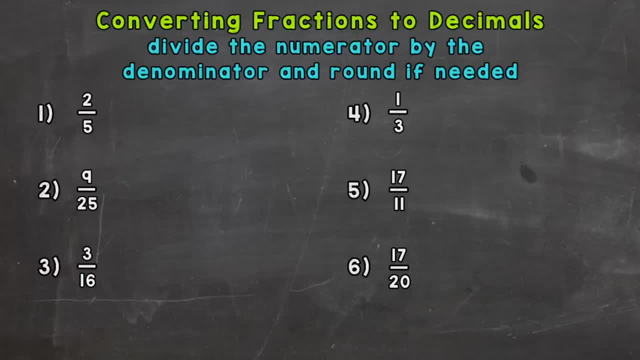 divide the numerator by the denominator, So two divided by five, And this fraction is less than a whole. So our decimal is going to be less than a whole as well, because this decimal is going to be equivalent to two-fifths. So we can't do two divided by five, right? We can't take a whole.